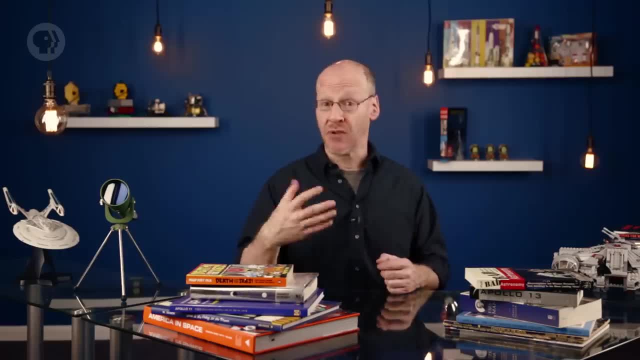 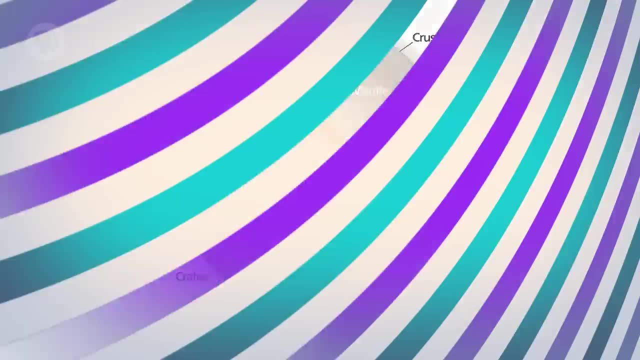 satellite is a lot smaller than you think. The internal structure of the Moon is roughly similar to the Earth. It has a solid iron inner core, a liquid outer core, a thick mantle and a crust of lighter material on top. The core is small, probably 350 kilometers in radius, and still hot, though not as hot. 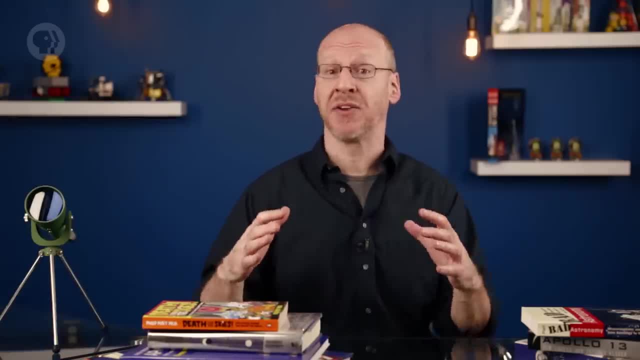 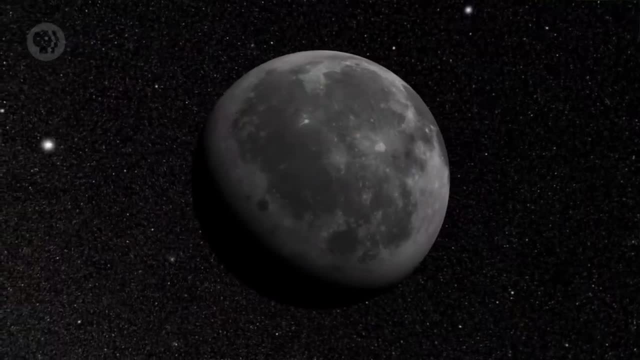 as Earth's core. The lower mantle may be a thick fluid, but unlike Earth's mantle, the upper part is solid. The easiest part of the Moon to observe is its surface, so of course we know the most about that. The near side, the side we see from Earth, is divided into two distinct types of regions. 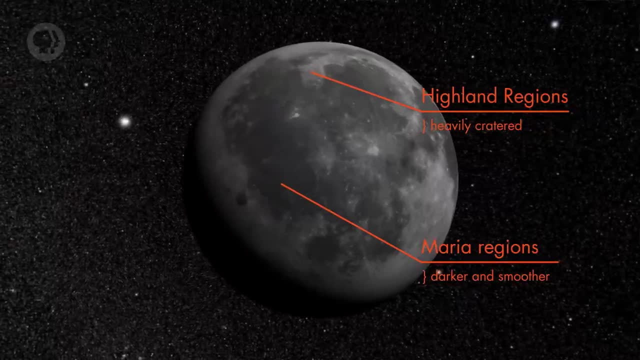 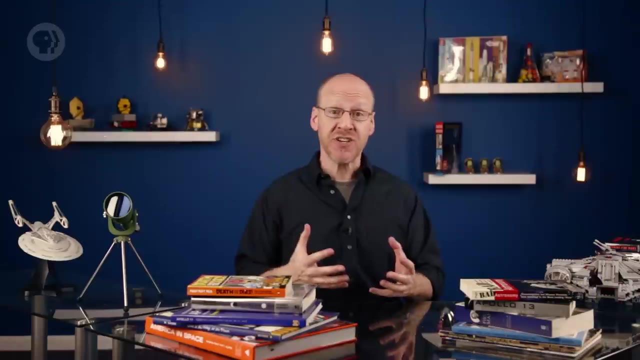 — highlands, which are heavily cratered, and maria Latin, for seas which are darker and smoother. The craters in the highlands are from countless impacts over the eons from asteroids and comets. Rocks from these regions have been dated to be well over 4 billion years old. — nearly as old as the Moon itself. The maria, on the other hand, don't have nearly as many craters. They're younger, but that's relative. Rocks from those areas appear to be roughly 3 to 3.5 billion years old on average. 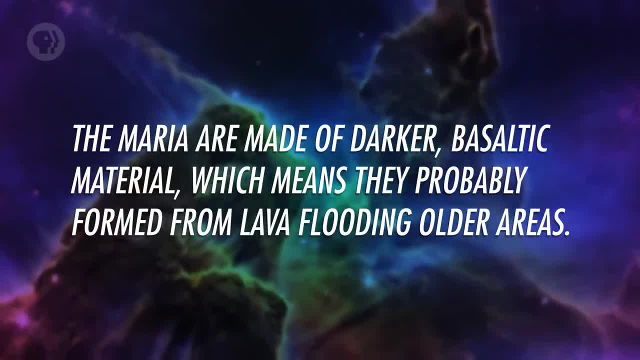 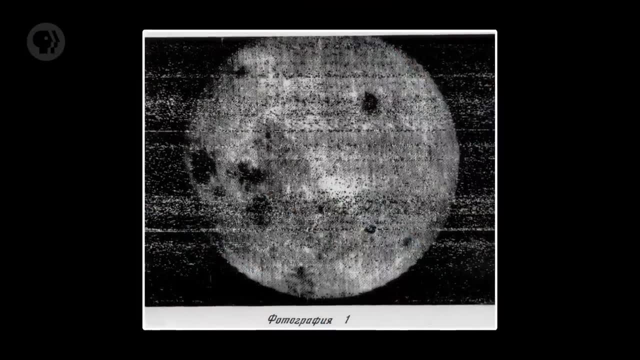 The maria are made of darker basaltic material, which means they probably formed from lava flooding older areas. For most of human history the far side of the Moon was hidden from us, But in 1959, the Soviet Union flew the Luna 3 space probe around the Moon, photographing the far side. 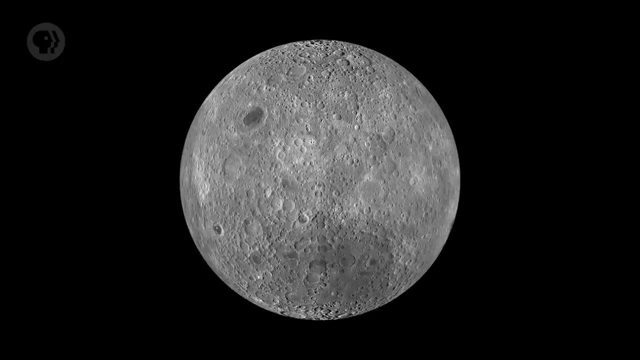 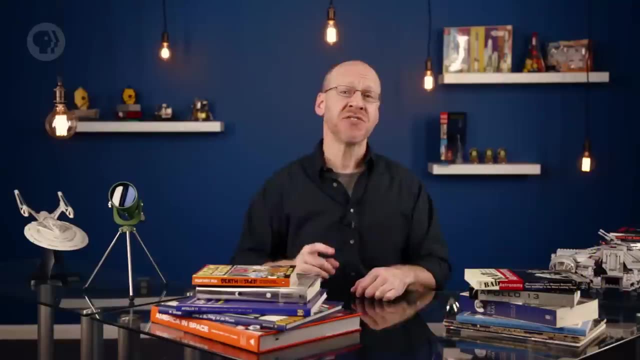 for the first time. Everyone expected it to look a lot like the near side, but shockingly it's vastly different. There were almost no maria. That's weird. The near side is covered with them And they're not. And not only that: observations from subsequent lunar probes showed the crust on the lunar 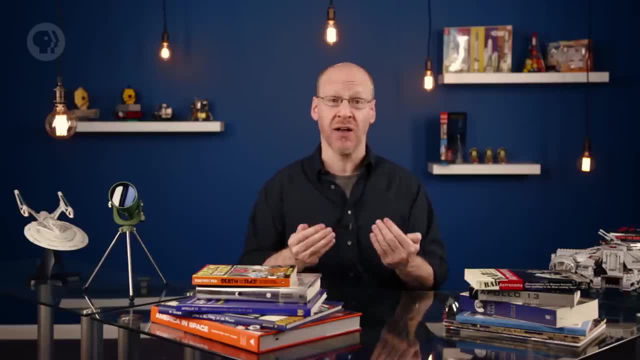 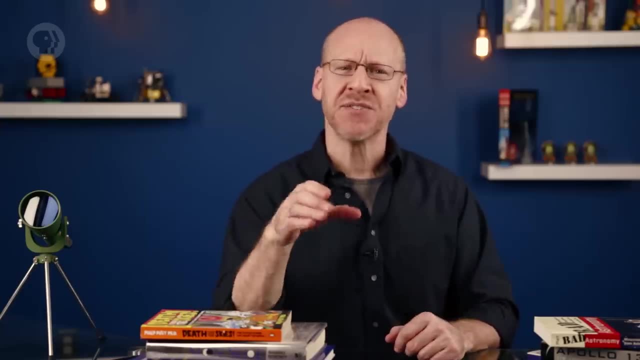 far side is thicker than it is on the near side as well. The Moon is starting to stack up mysteries. Why is it so big compared to Earth? Why are the near and far sides so different? It turns out the composition of the crust has a lot. 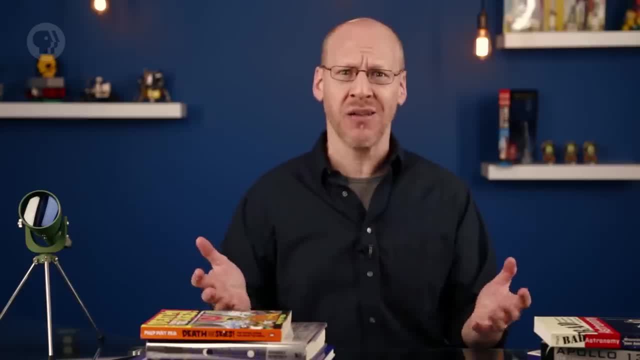 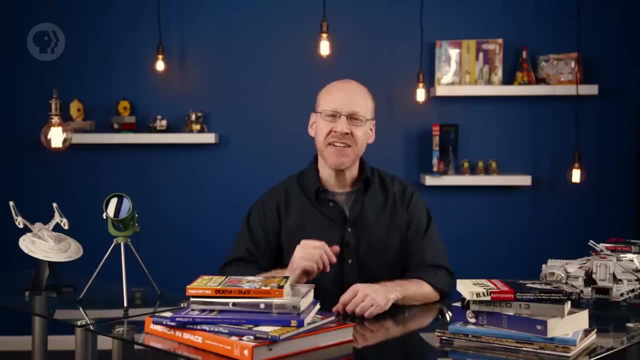 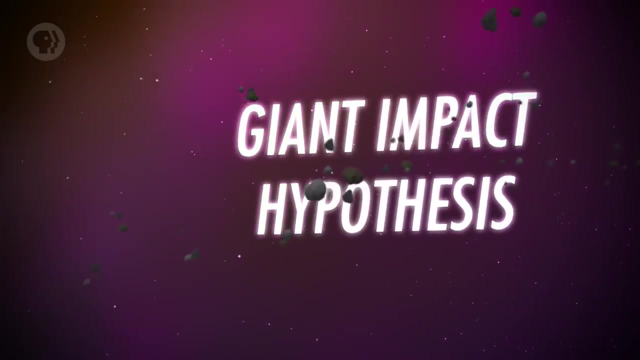 of similarities to Earth, but also a lot of differences as well? Why It turns out? the answers to these questions are all related to how the Moon formed 4.5 billion years ago, But the best one going these days is called the Giant Impact Hypothesis. When the solar 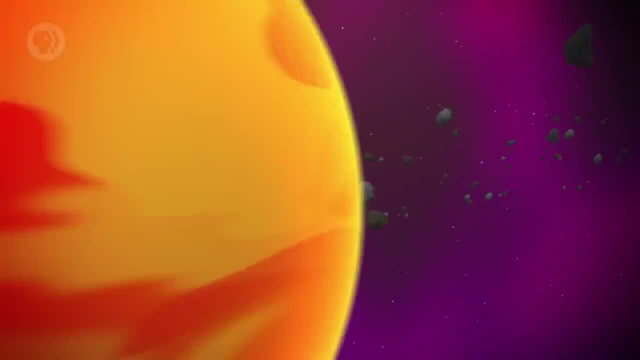 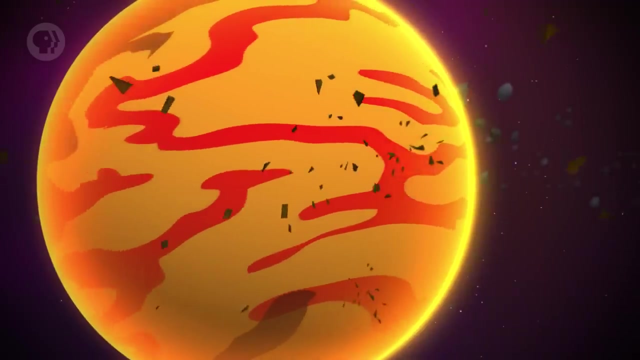 system formed, there were a lot more objects orbiting the Sun than there are now. These ranged in size from grains of dust up to objects the size of planets, And that meant there were lots of collisions. No doubt the Earth suffered many such impacts, But one happened late in Earth's history. 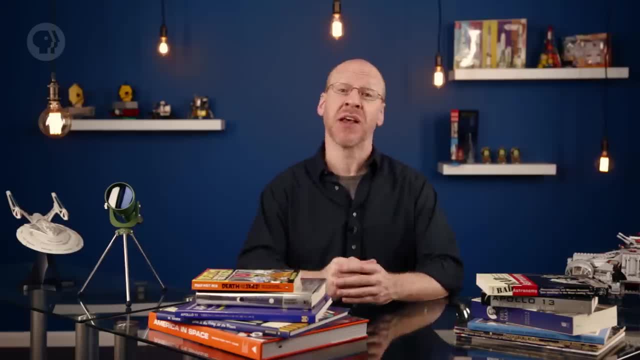 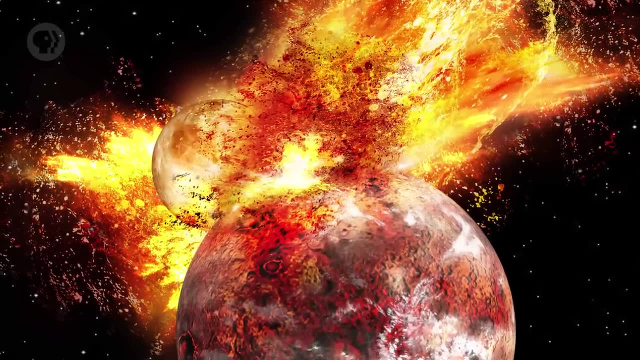 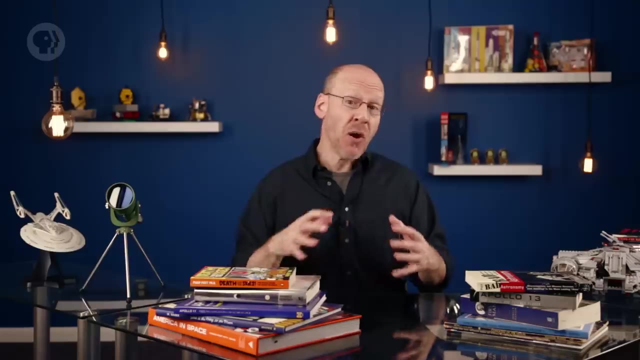 relatively speaking. roughly 50 million years after things started to settle down, A Mars-sized planet given the unofficial name Theia slammed into our young planet. But it wasn't a head-on impact, It was a grazing collision. The impact was colossal, blasting a huge amount of material from both planets into space. Most, 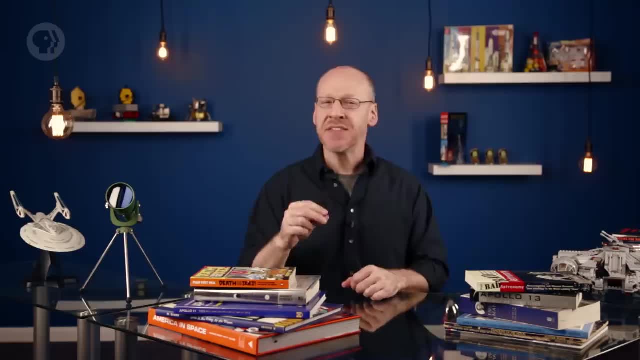 of it came from the outer layers of the Earth. since the collision was a grazing one, This material rapidly coalesced into the Moon, and that explains why there's some- but not total- similarity in composition to Earth. It used to be part of the Earth. 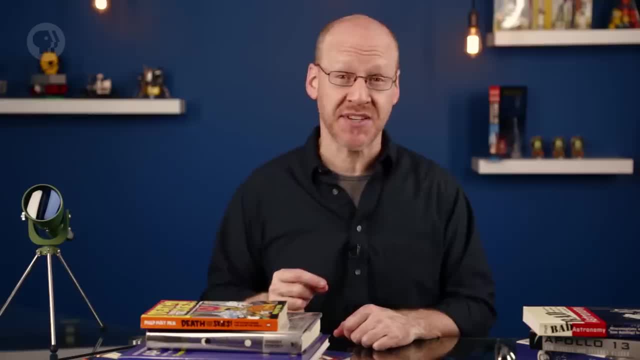 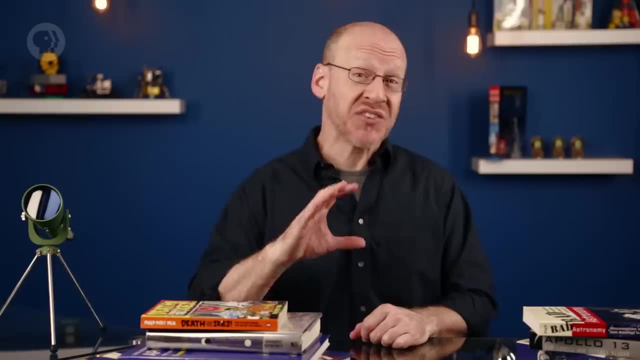 But some of it came from the other planet too, And we may even have some evidence of it. Some rocks from the Moon show a peculiar ratio of different kinds of oxygen atoms, called isotopes. It's possible some of the more exotic isotopes of oxygen came from the other planet. Actually, this idea has been around for a long time, ever since the Apollo missions in the 1970s. There's a lot of evidence to support it too. But a new twist on it goes farther. When the Moon formed from the debris of the collision, it was close to Earth probably. 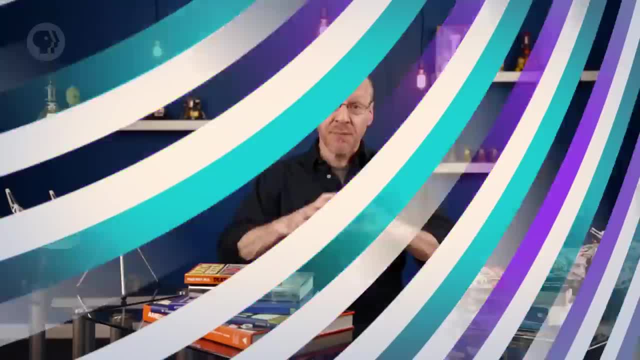 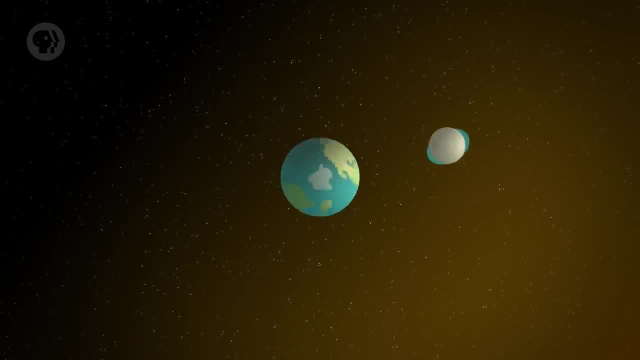 20,000 kilometers away. The collision was so violent that it completely melted the Earth and the Moon was molten too. Tidal forces rapidly synchronized the Moon's spin and orbital period so that one face always pointed to Earth. The collision was so violent that it completely melted the Earth and the Moon was molten too. 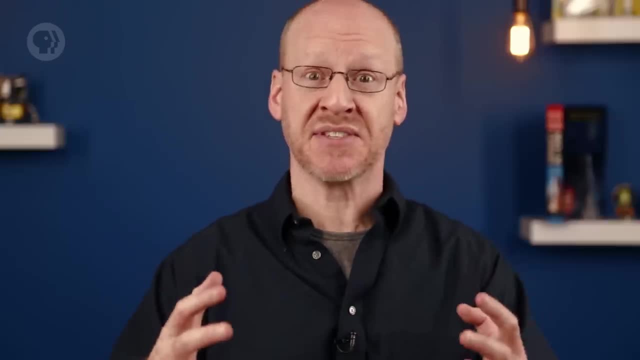 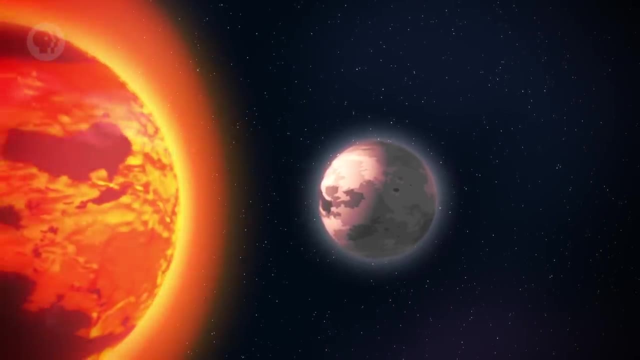 If you were on that side of the Moon, the Earth would dominate the sky, appearing 80 times larger than the Moon appears in our sky today. And the Earth was hot. It hung there like a blast furnace and would have seriously heated the near side of the Moon. 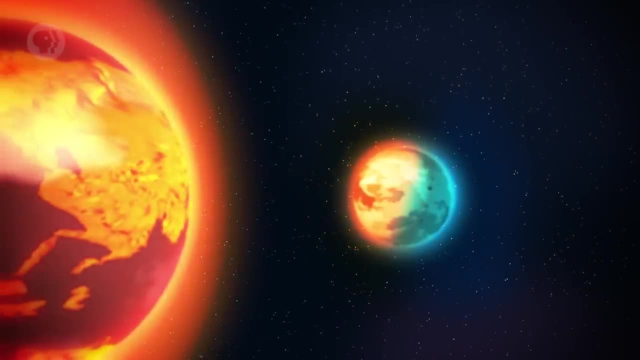 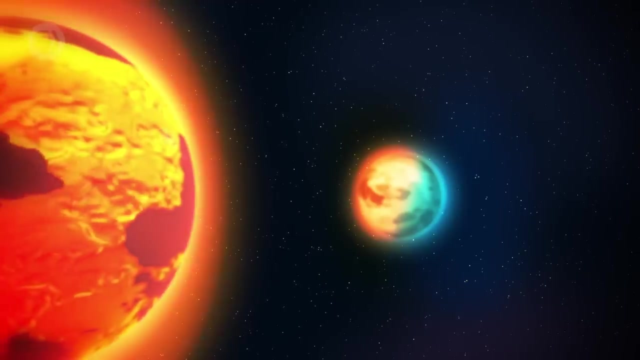 The far side would have been much cooler. The material on the near side would have vaporized and a lot of it would have condensed on the far side Over time. this created the thicker far side crust we see today. Then there was another seriously terrifying event: the Late Heavy Bombardment, a period 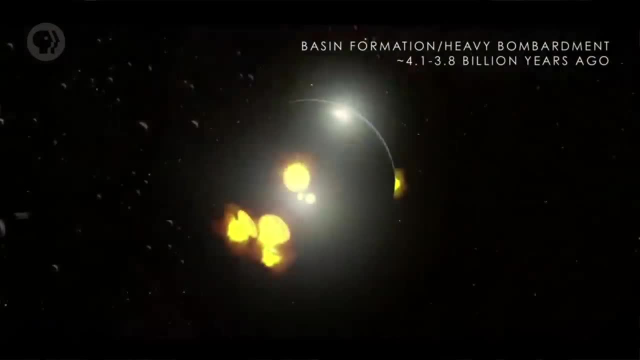 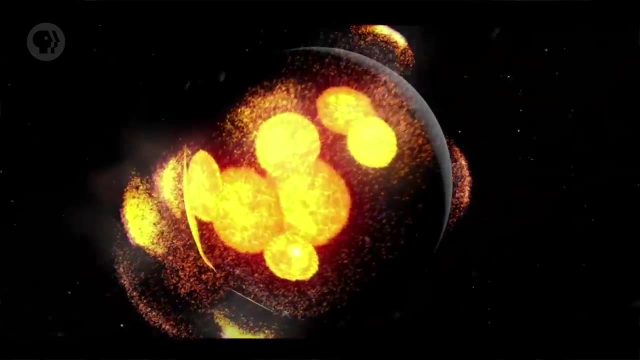 of intense collisions with comets from the outer solar system, probably triggered by the movement of outer planets. This rain of millions of comets left scars on all the inner worlds, including the Moon. That's when most of the highland cratering occurred. Some of these collisions were massive, carving gigantic craters on the Moon. Later, lava bubbled up through cracks in the Moon's surface, flooding these craters, creating the maria we see today. Ah, but the far side's crust was thicker. Impacts there couldn't get as deep and it. was harder for lava to break through and bubble up. That explains why there are so few maria there. This idea that the Earth cooked the Moon and formed the crustal anomaly is pretty new and is still being argued over. There are also competing hypotheses about this as well. 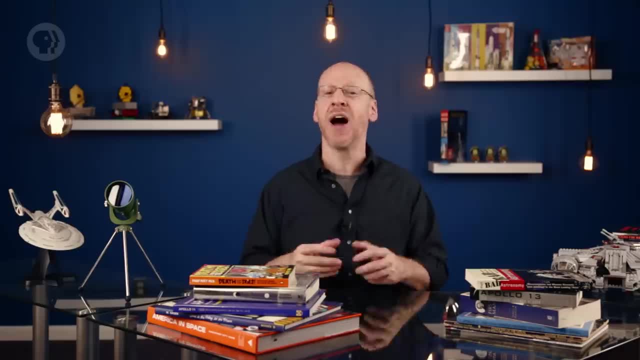 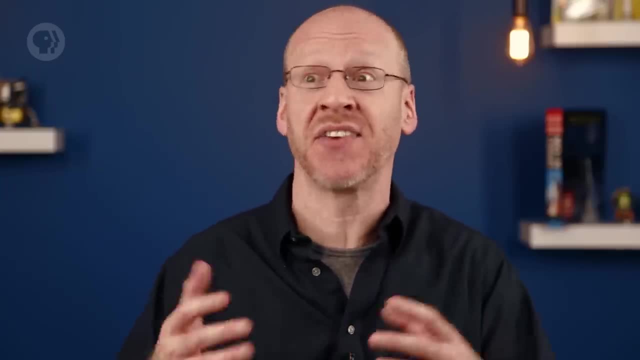 As we gather more evidence, we'll eventually get a better understanding of just why the Moon's crust is so weird. After all that, I have to say, it's a little unfair to divide the lunar surface today into just highlands and maria. 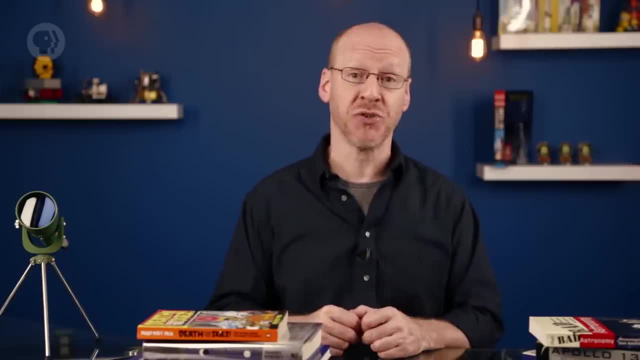 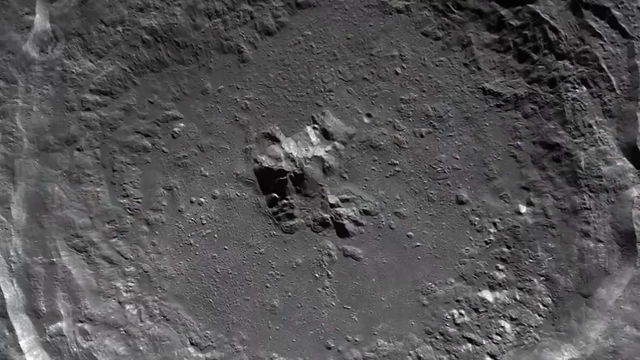 For example, craters are pretty diverse. Some are small, in simple bowl shapes, Others are huge, dozens of kilometers across and more punctuated, with a central peak, A mountain in the middle that formed as material from the gigantic impact that formed it splashed. back up in the middle, Double craters are common too, probably formed when binary asteroids hit the Moon. There are also crater chains, long lines of small craters that may have formed when a nearby large impact splashed out long streamers of material. 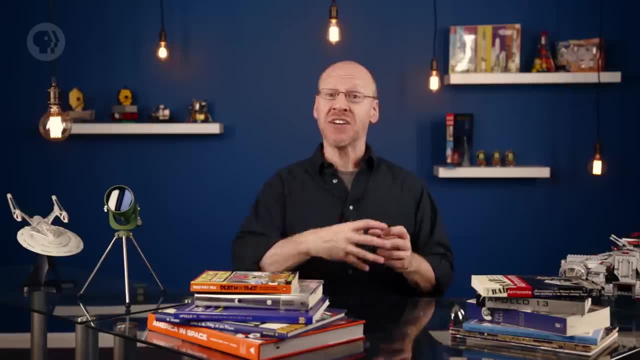 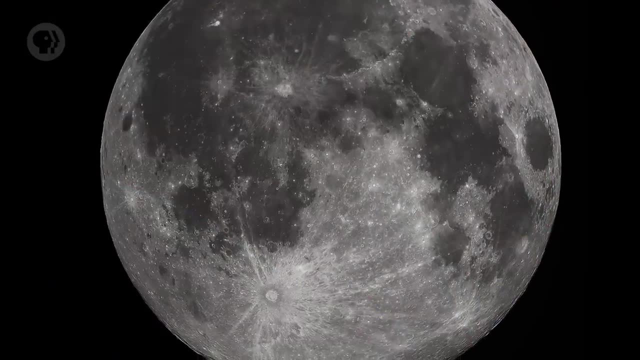 Rays are common from big craters too. These are extremely long splash marks pointing radially out from the impacts. These are extremely long splash marks pointing radially out from the impacts, probably from the moon. They were probably formed when plumes of material were ejected. Some of the brightest are from: 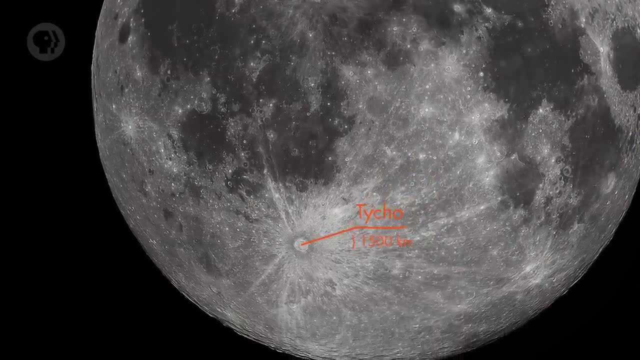 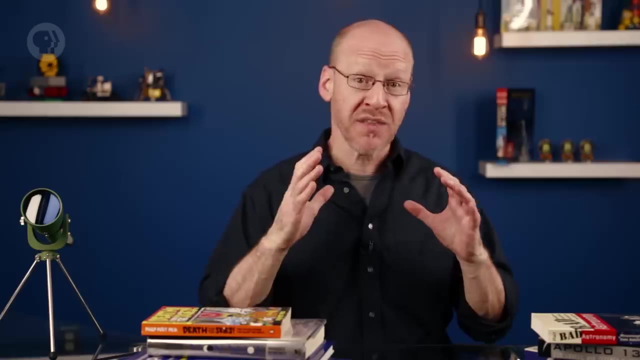 the crater Tycho in the Moon's southern hemisphere, and they stretch for 1,500 kilometers. The material is a bit more reflective than the surrounding terrain, so they appear bright in contrast and are one of the most outstanding features visible near the time of the full. 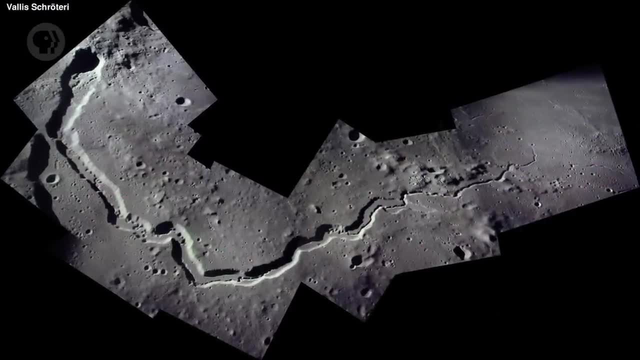 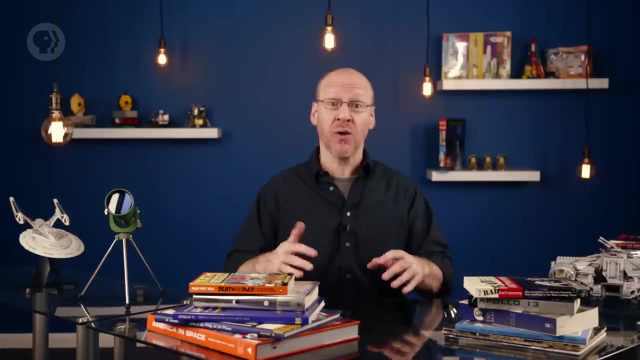 moon, And there's so much more. Long sinuous rills like dry riverbeds wind their way across the surface, actually the sites of ancient lava flows. There are lava tubes as well, where the top of a lava flow cooled and formed a torrent. 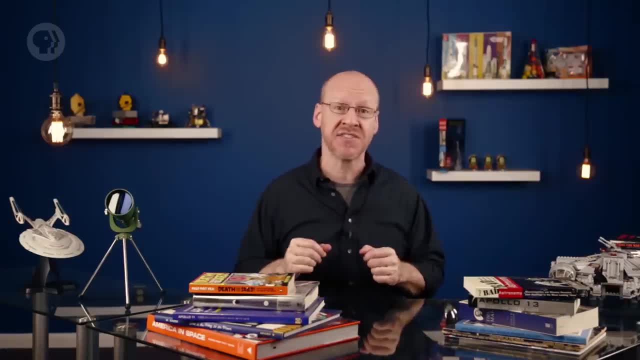 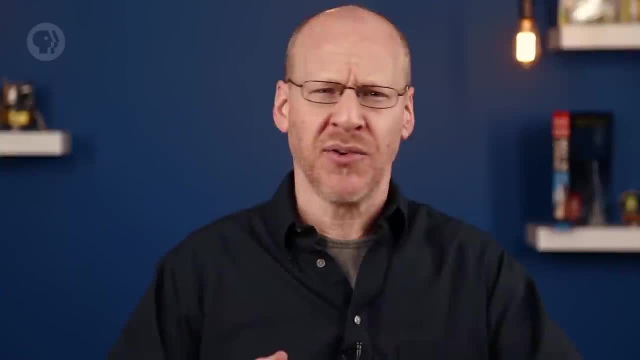 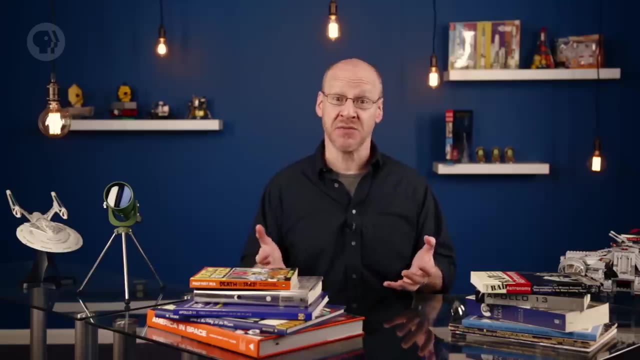 Sometimes the roof, as it's called, collapses and forms a skylight and we can see into the otherwise hidden tunnel. There are also cliffs, mounds, ancient and quite dead volcanoes, even mountain chains. There's no tectonic activity on the Moon, but mountain ranges formed at the edges of 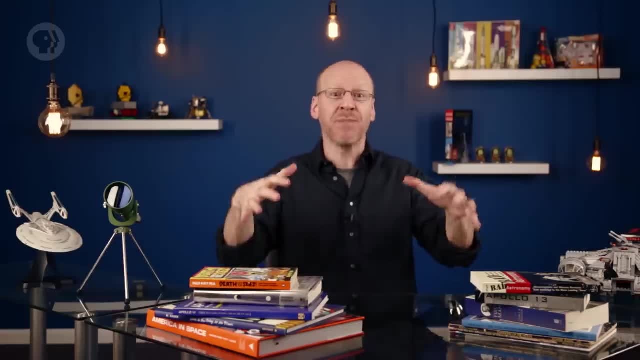 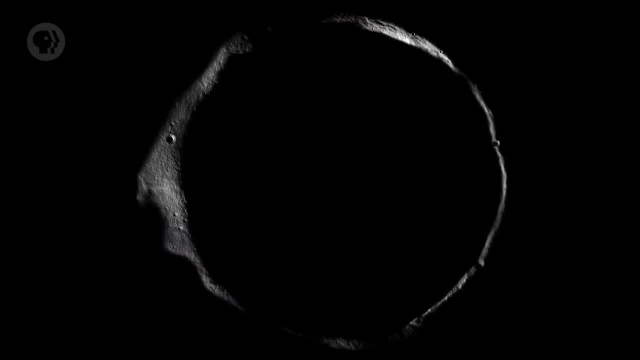 giant impacts where the huge forces unleashed pushed up the rocks at the crater rim, And new observations show there's something else on the Moon too. Water Deep craters near the Moon's poles have floors that never see sunlight. Comet impacts can distribute. water all over the Moon, but most of it is destroyed by sunlight. But it can collect in these dark craters And studies show there could be over a billion tons of water there in the form of ice. That would be a huge boon to colonization. Water is heavy and really expensive to transport. 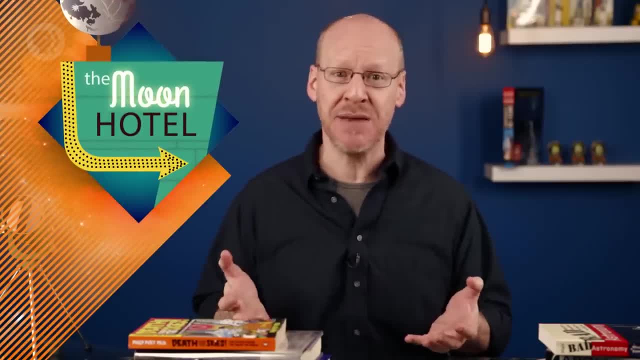 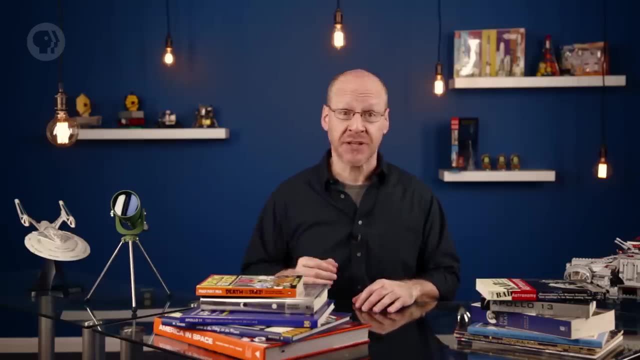 from Earth If it's already on the Moon. that makes it a lot easier to put people there And that's in our future. I have no doubt We're starting to get serious about going back to the Moon. NASA has plans of returning and other countries like China and India are looking moonward. 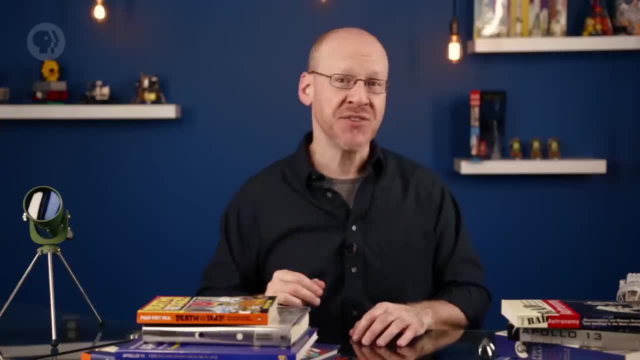 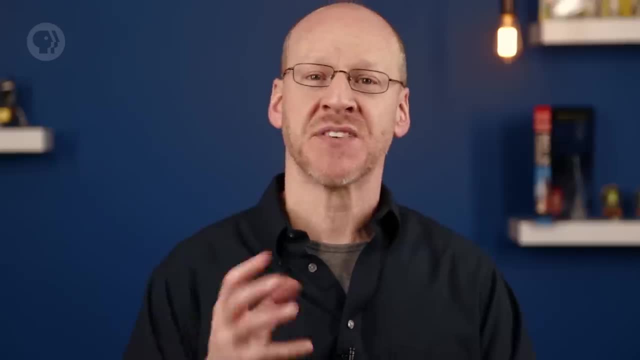 as well. It's not a matter of if, but when, And it could be soon, so soon that I bet there's a really good chance the next person to step foot on the Moon is already alive. Perhaps some teenage student in some country is just now taking an interest in science, math, engineering.